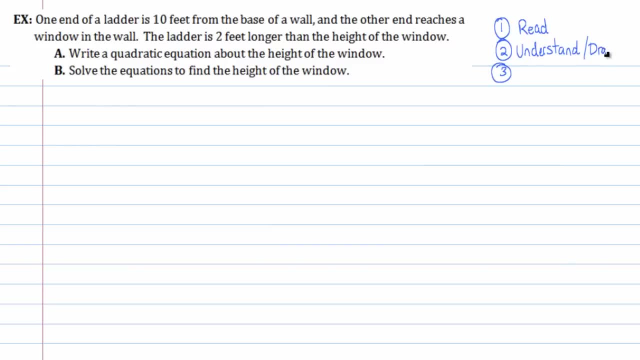 Generally, when you go for understanding what's going on, you should also draw a picture, if you can. So let me go ahead and draw a picture of this situation. We have a wall, so I'll just say that's our wall, right there. 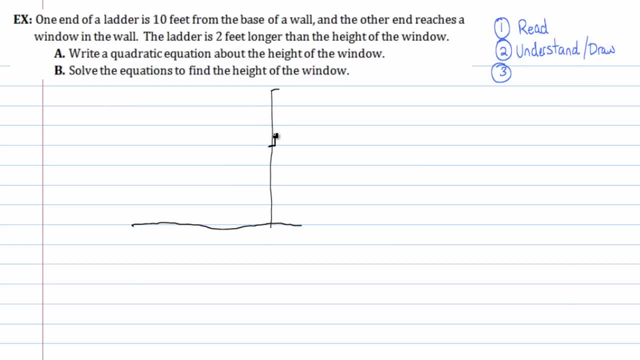 And we have a window set into the wall. let's just pretend that this is our window right here, And so let me make sure that this looks like a wall- Not the best wall in the world, but whatever- And we have a ladder. 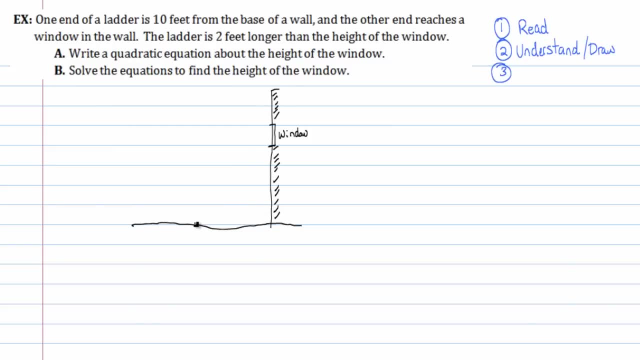 Where one end of it is ten feet away from the wall. So let's just, in fact, maybe I'll use a different color for the ladder- And one end is ten feet from the wall and the other end reaches the window in the wall. 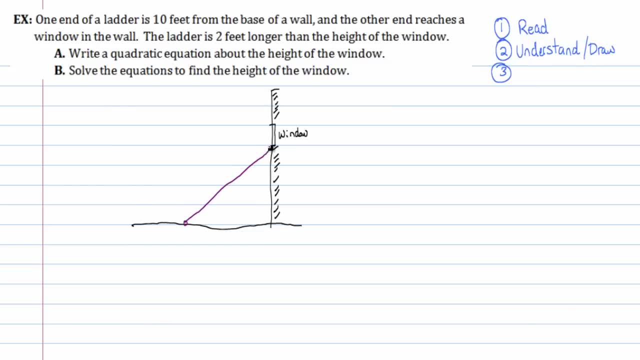 So it's this situation right here where you have a ladder leaning up and somebody's going to climb up this ladder to reach the window. Now there's something to be mentioned here that's not in the problem, but it's usually implied in the problem. 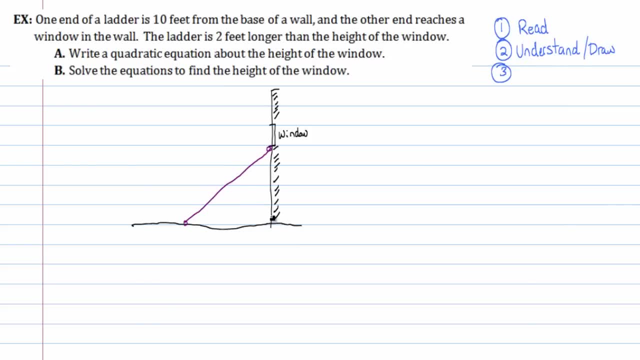 Nobody makes. unless you're in Italy, nobody makes a building that leans And, honestly, the Leaning Tower of Pisa wasn't made to lean okay, So this should be a right angle. That's kind of an implied piece of information. 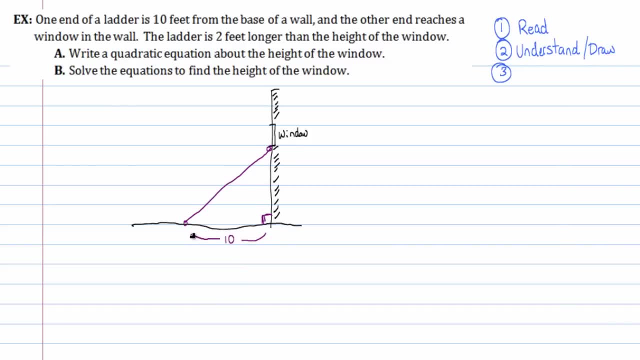 We know that this distance right here is ten feet. I should probably put the units mark in there: ten feet And the ladder is two feet longer than the height of a window. Write an equation about the height of the window. So we need to find the height of the window. 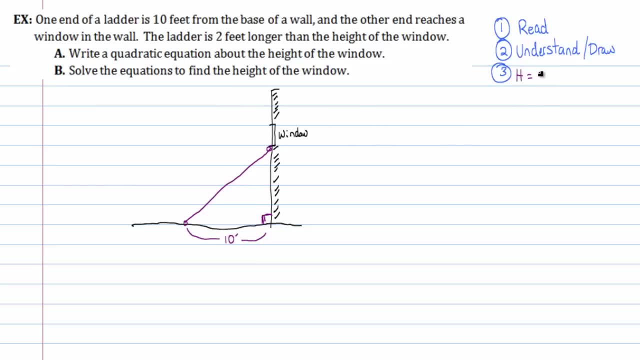 I'm going to label. I'm going to label the height as h, So h equals height of window And I'm a big fan actually of labeling all my unknowns. So if h is the height of the window, 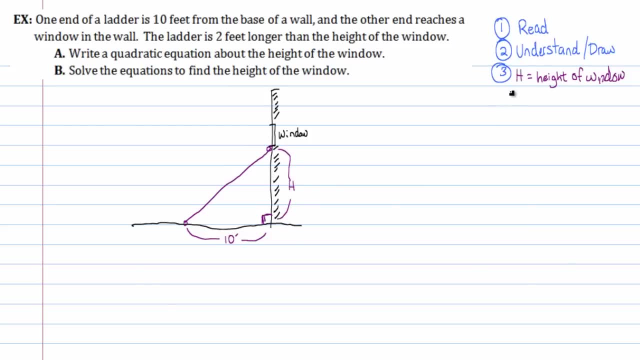 the other thing we don't know in this situation is the length of the ladder. L is length of ladder And I know that most instructors teach this to just kind of read this and immediately fill in the length of the ladder. But the reason why I like to take my time with it, 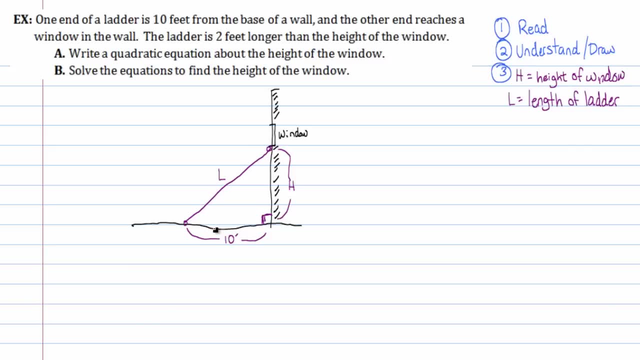 is because I want to introduce- or actually you've already been introduced to it- solving systems of equations. This is essentially going to be a system of equations. So now that I have this kind of set up like this, I can find a relationship between the variables and the number ten. 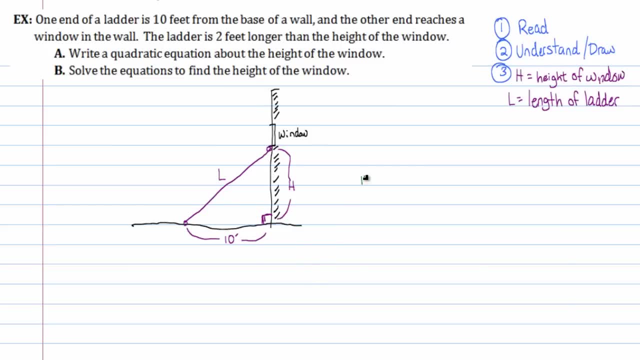 The relationship is the Pythagorean Theorem: Side squared plus other side squared should equal the hypotenuse squared. That's for a right triangle only, And of course I have one equation and two unknowns, So I need another equation. 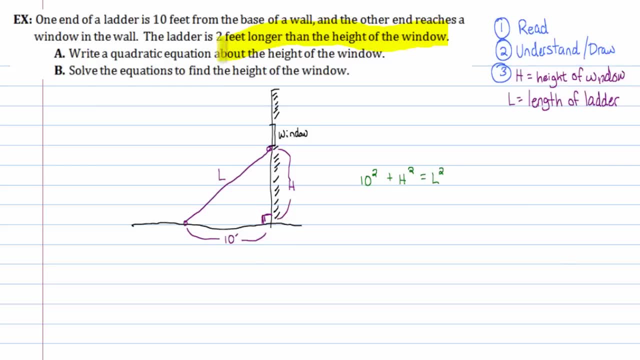 And that will come from this second sentence. here The ladder is two feet longer than the height of the window. So in other words, L is two feet more than the height of the window. Wherever I see an L in this previous equation. 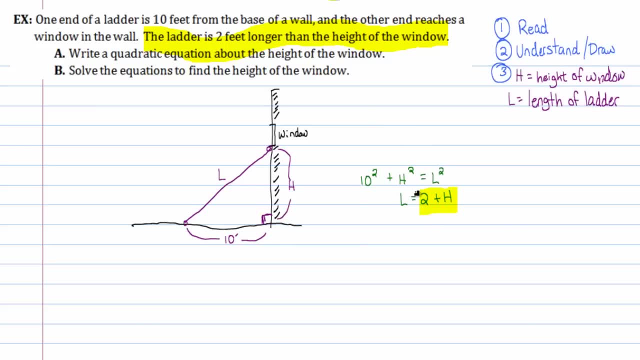 I'm going to replace it with two plus H. So that's what I'm going to do, So I get one hundred plus H squared will equal two plus H being squared. That's a quadratic equation about the height of the window. 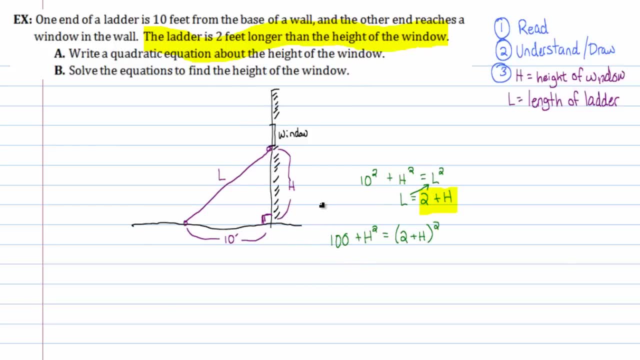 And now the second part is just asking me to solve the equation. It says equations. It should be just equation. Uh, What's the equation? to find the height of the window. Okay, I see that I have to clean up the right-hand side. 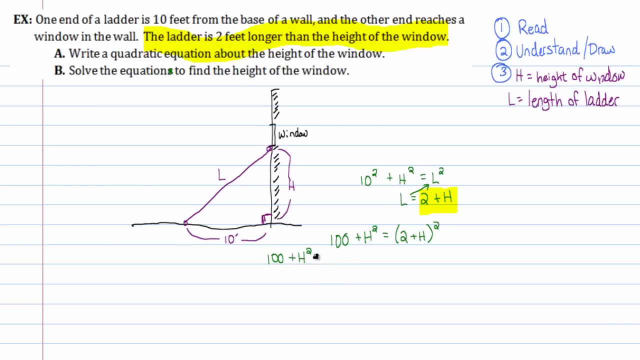 So at this point I generally forget about the word problem And I just concentrate on the mathematics here, the mathematical sentence. Remember that the quantity two plus H being squared means two plus H times two plus H. I will distribute the two through and the H through. 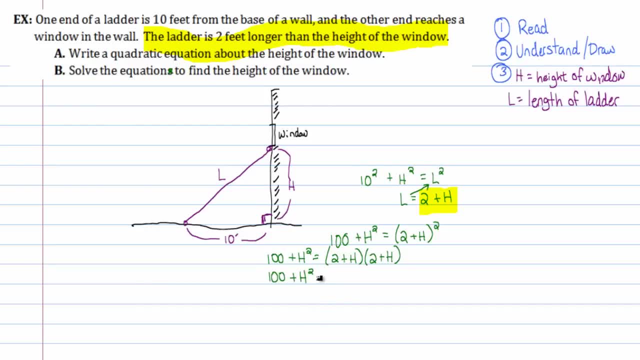 And when you do that you get this beautiful one hundred plus H squared is equal to four plus four, H plus H squared. Now initially I think, oh, there's two different versions of my variable And technically there are sitting here two versions of H. 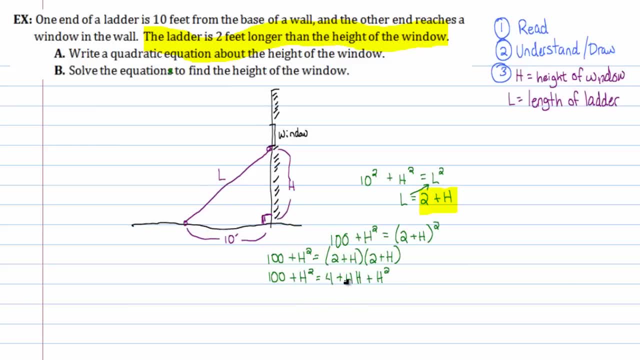 There's a single-powered version and a double-powered version. However, have some forethought here. Be able to look ahead a little bit And notice that when you subtract H squared from both sides, they'll cancel out nicely And you'll get this wonderful equation. 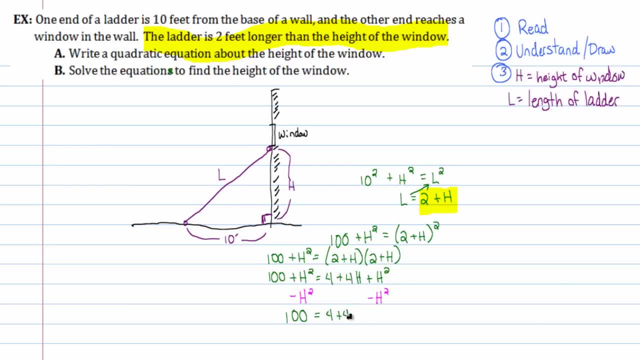 One hundred is equal to four plus four H. Now that I only have one version of my variable, I don't have to move everything to the right-hand side. I can just start solving for H. So I'll subtract four from both sides. 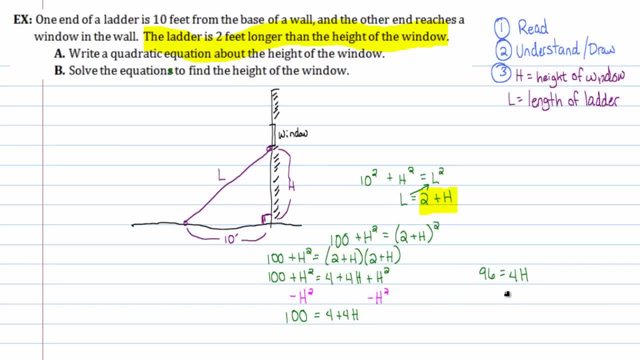 to get that ninety-six is equal to four H, And then divide both sides by four, H is equal to twenty-four. And remember, we want to find the height of the window. We've just found it: The height of the window is twenty-four feet. 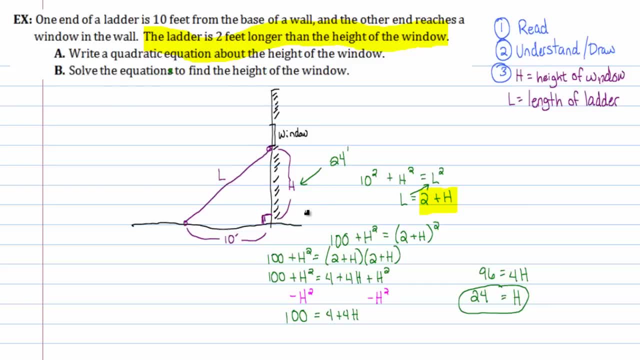 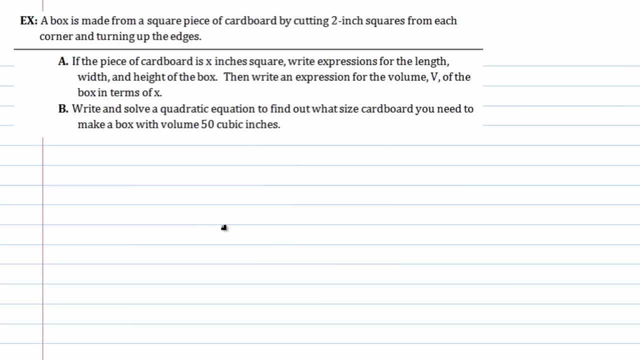 Remember we're dealing with units in feet. By the way, if somebody asks what the length of the ladder is, it's just two feet longer than that. The ladder is twenty-six feet. The next example here is that we have a box made from a square piece of cardboard. 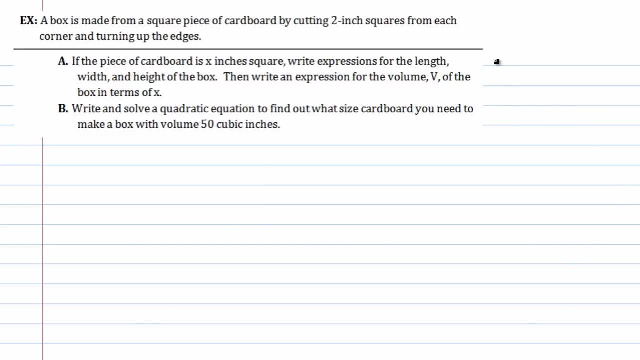 And, of course, you're given a square piece of cardboard. you can cut out these corners, And so let me draw a picture of that so you can kind of see If you have a square piece of cardboard here. not the perfect drawing. 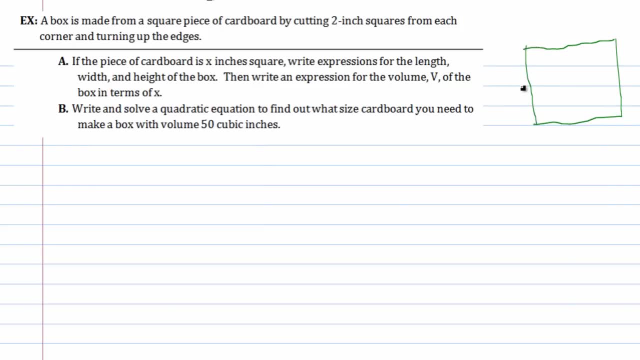 but good enough, it'll do. You can cut out corners. Cut out this corner, cut out this corner, and so on and so forth. When you do that, it allows you to fold up those flaps and you get an open box. 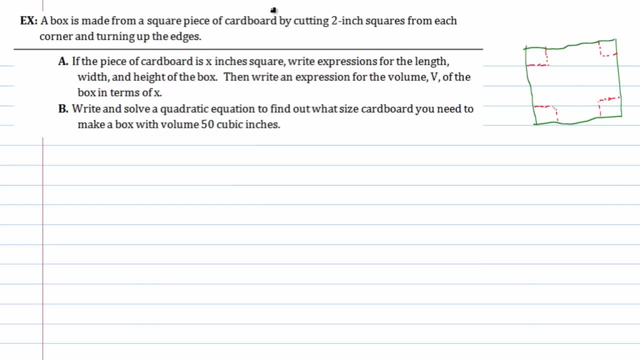 So I just wanted to kind of show you that picture. You can form a square piece of cardboard by cutting two-inch squares from each corner and turning the edges up. So these are two-inch squares. Alright, you get the idea. I don't need to do the whole thing. 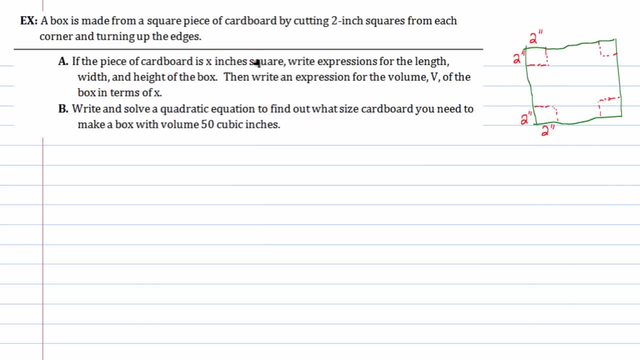 If the piece of cardboard is x inches square, which means that the length here is x inches. So the length here has to be x. So the length here has to be x inches as well If the cardboard is x inches squared. 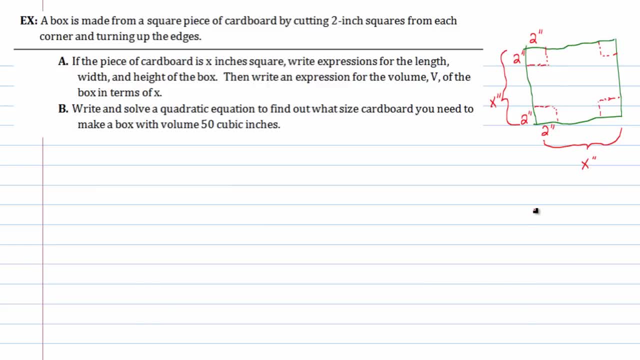 write expressions for the length, width and height of the box. Oh well, Let's see The length of the box. we'll call that L is equal to. Now, of course, when I write L is equal to. 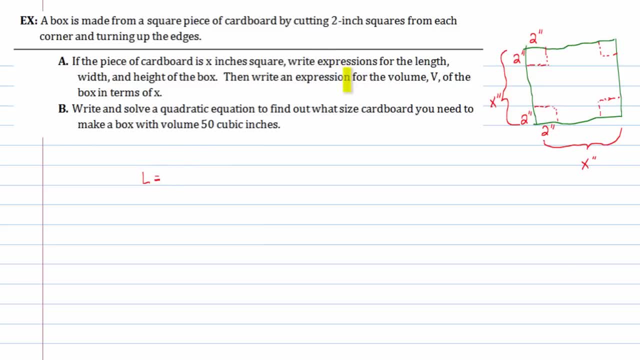 I really shouldn't do that. They're asking me to write an expression, not an equation, but an expression, So maybe I shouldn't write: L is equal to here. Maybe I'll instead go ahead and just write an expression. The length is just going to be this length: x. 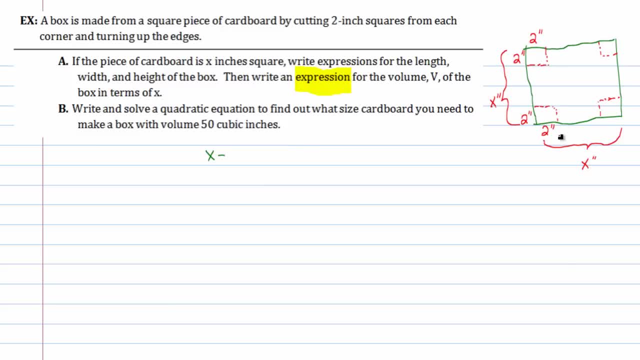 but we lose some of that length When we fold up the edges. we lose two inches because it's rightmost edge and two inches because it's leftmost edge. So the length- here, the expression for the length, it's going to be x minus four. 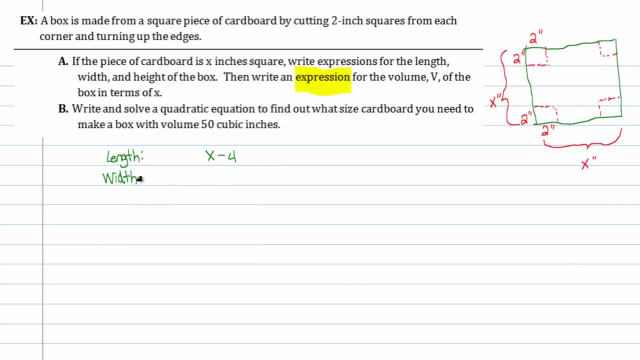 The expression for the width. again, just using some logic here, The width- let's see the whole width- is x of the cardboard square, but we're losing two inches top and bottom. so that's the width. The height of the box, though. 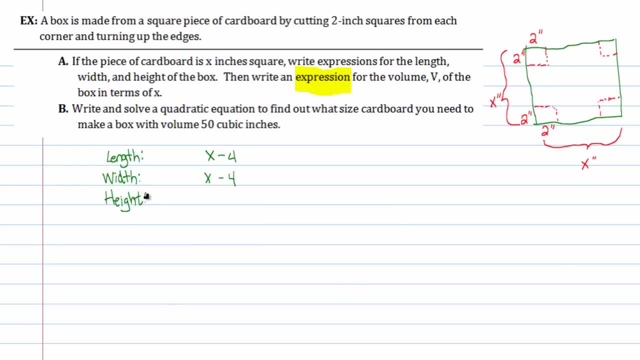 is kind of interesting, The height. well, if you fold up these corners, they're only two inches tall. The height is only two inches. Now write an expression for the volume. Well, volume is just length times width times height. 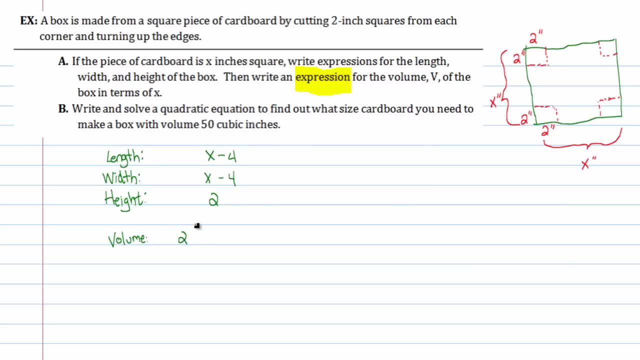 That's for a box. Volume is length times width times height, So that's two times x minus four, times x minus four. And let's see part B: write and solve a quadratic equation to find out what size cardboard you need. 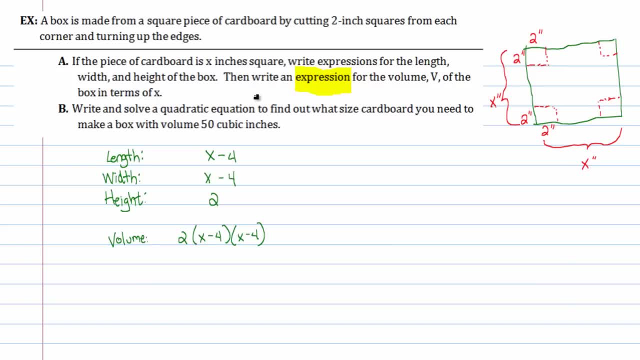 to make a box with volume 50 cubic inches. So part B here is just asking us: hey, how can that volume be 50 cubic inches? In other words, I want this volume expression here to be 50.. And remember, I cannot just say: 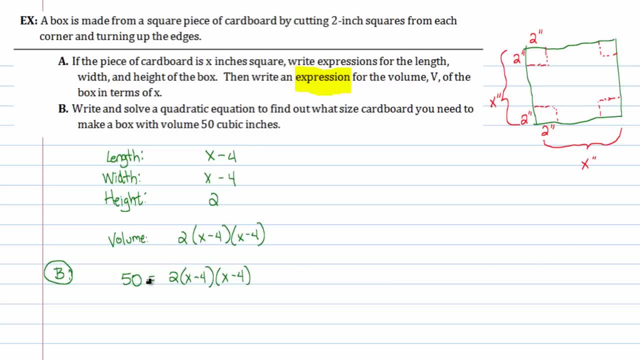 oh, therefore x minus four is equal to 50, or x minus four is equal to 50. I can't do that. What I have to do, actually, is distribute the x minus fours into each other, So in other words, multiply those two binomials. 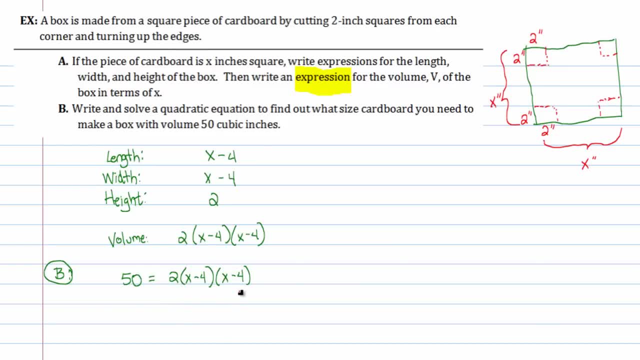 I'm going to do a little trick first. You don't actually have to do this, but I'm going to divide both sides by two, just so that these two cancel and I get 25 over there. You don't have to do that. 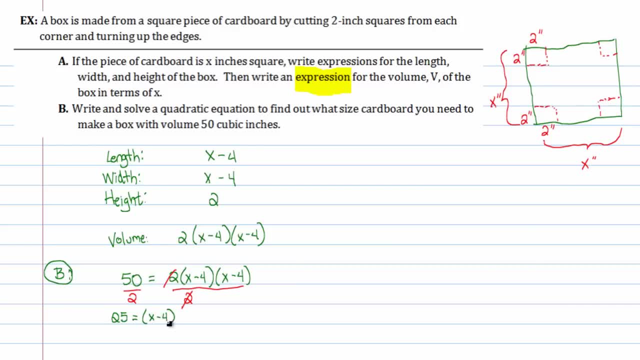 I'm just doing it to kind of make my life a little bit easier during this process. Let's distribute through on those binomials So you should get: 25 is equal to x squared minus eight, x plus 16.. And let's subtract 25 from both sides. 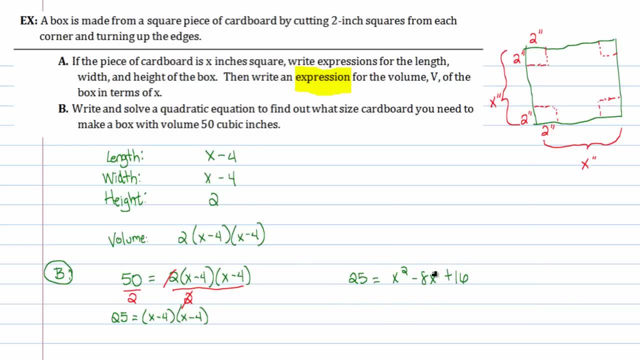 because, see, we have an equation with two different powered versions of our variable, So we have to move everything to one side. So I'll subtract 25 from both sides. I get this business here. 16 minus 25 is negative nine. 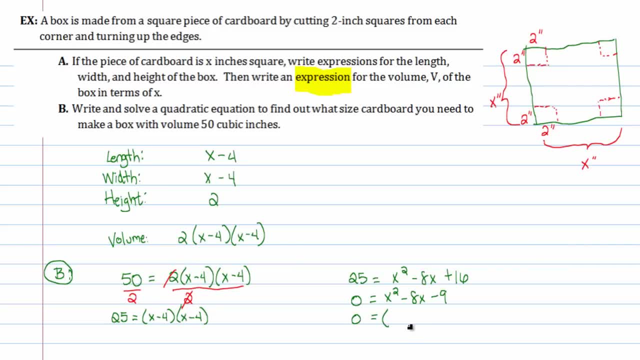 And hopefully that factors. It actually does. It factors to x minus nine times x plus one. So this means that either x is equal to nine or x is equal to a negative one. Think about this: X is a length, right. 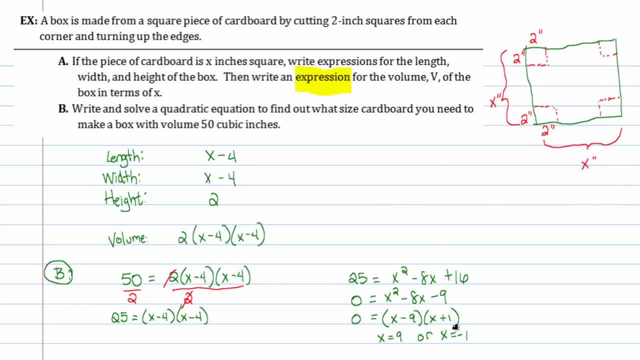 It's the length of this cardboard. So one of these solutions does not make sense, and that's often the case in physical situations- That when you're solving a quadratic equation that dominates or describes a physical situation, one of the solutions likely is going to fall out. 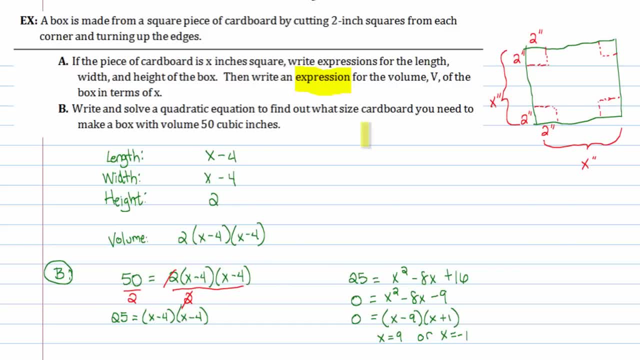 It's usually the negative solution. Not that all quadratic equations have a positive and negative solution, but often it happens when you're solving applications. So our real answer is: x equals nine. So the size cardboard will need is a nine inch by nine inch. 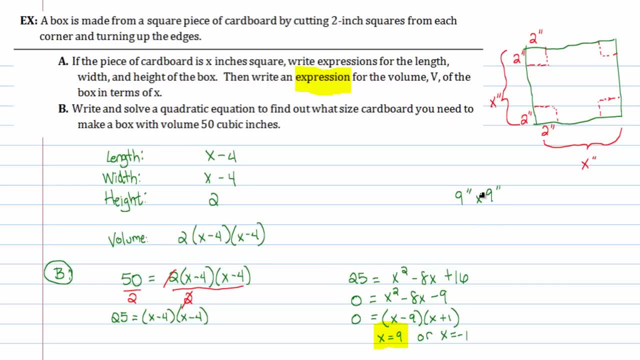 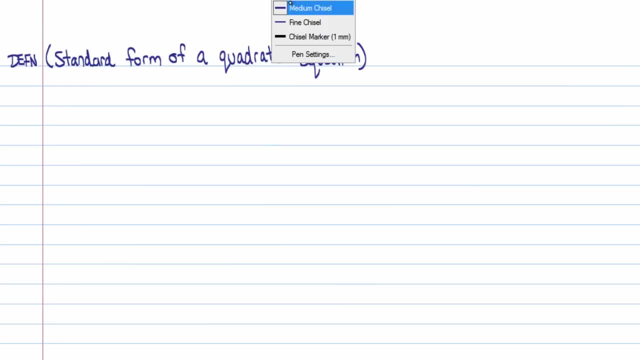 Or in other words, 81 square inch piece of cardboard. Now, before I do my last example here, I want to introduce another definition, And this definition is needed for the next example. Standard form of a quadratic equation. The standard form of a quadratic equation is this: 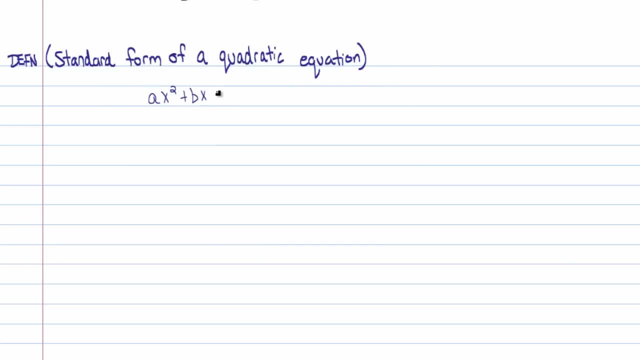 A, x squared plus B, x plus C is equal to zero. That's what they call standard form. So you have an equation in x here and it all equals to zero. It's just necessary for the following example Examples: find a quadratic equation. 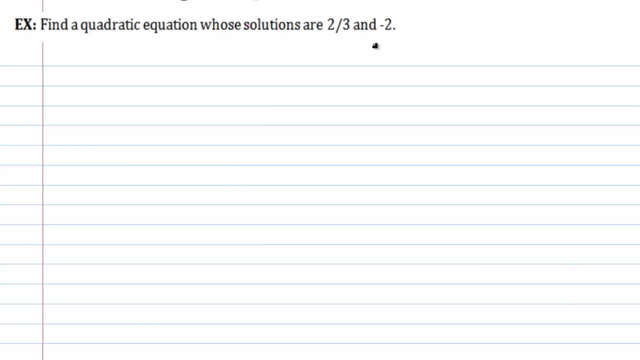 whose solutions are two thirds and negative two, And I'm going to tack on a little bit more- Written in standard form with integer coefficients. That's important for this example, because it's very easy- although you may not think so yet, it's very easy- to find the quadratic equation. 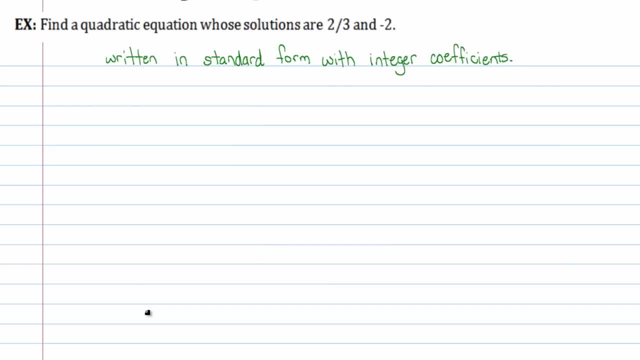 whose solutions are two thirds and negative two. In fact, if I told you I had a quadratic equation with solutions being two thirds and negative two, then you could say: oh, that means at the end of solving, you got the following: X equals two thirds. 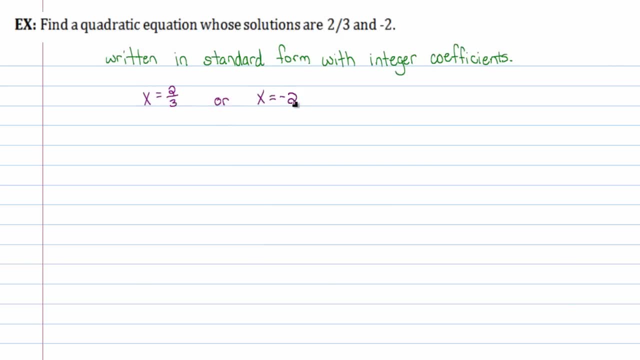 or x equals a negative two, And that would be true. Of course. you could then say: listen, actually, if I want to rebuild the quadratic equation that you got, that you were given so that you could have these solutions, I'm going to go ahead and basically move all values. 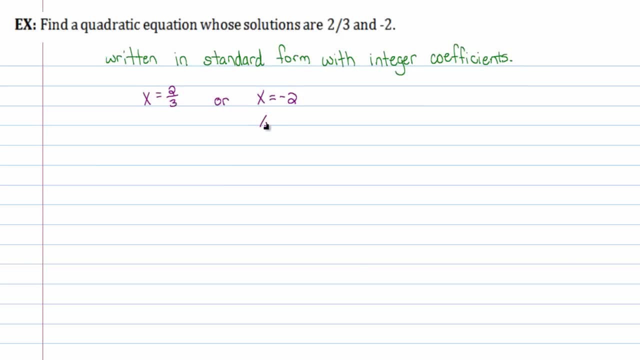 to the left-hand side. In other words, on this one over here, I'm going to add two to both sides, so I get x plus two. had to be zero. And on the right, on the left-hand side, I'm going to write this: 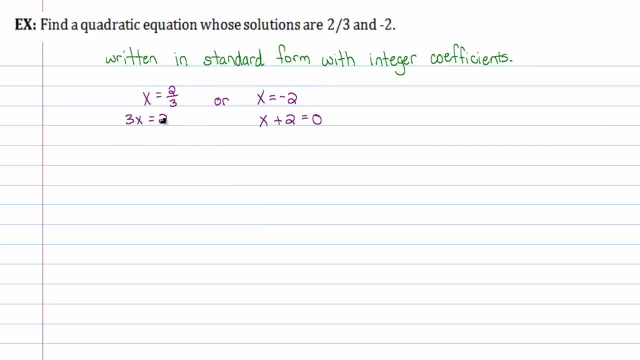 I'm going to multiply both sides by three, so I get three x is equal to two. That's an important step. Get rid of fractions. and then subtract two from both sides, So three x minus two is equal to zero. So these are the two objects. 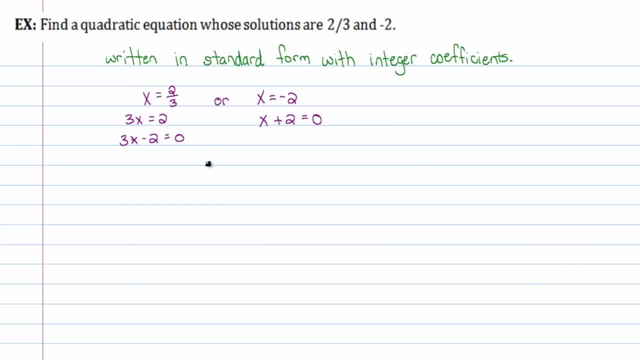 that must have been multiplying to become zero. This means that either three x minus two was zero or x plus two is equal to zero, Which means that when you multiply them well, the product has to be zero. In other words, three x minus two times x plus two has to be zero. 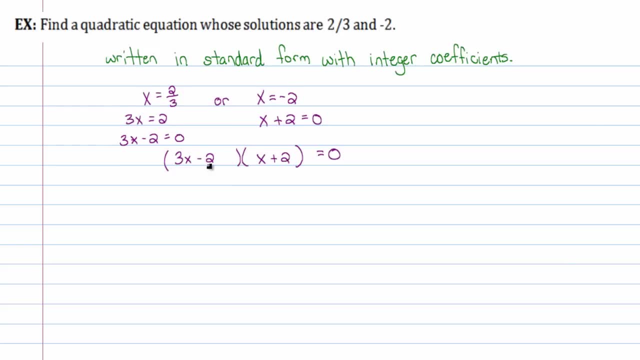 Well, we're almost done here. If you distribute through, in other words you multiply these two binomials together, you get the following: Three x squared plus six x minus two x minus four is equal to zero, Or in other words: 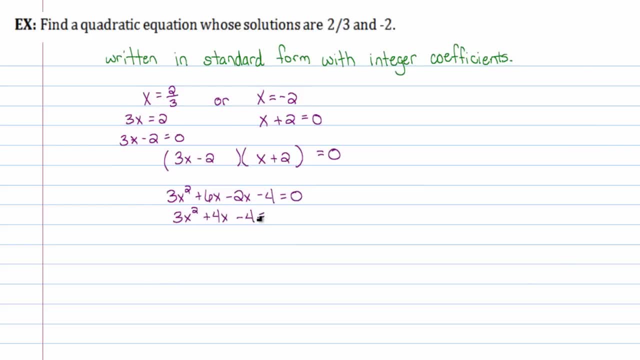 three x squared plus four x minus four is equal to zero. And lo and behold, I have a quadratic equation in standard form with integer coefficients. How did we do it? Well, notice in this problem-solving process. if I go back to maybe one of the previous examples here, 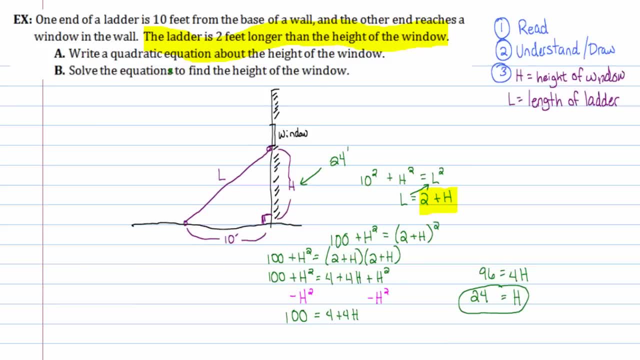 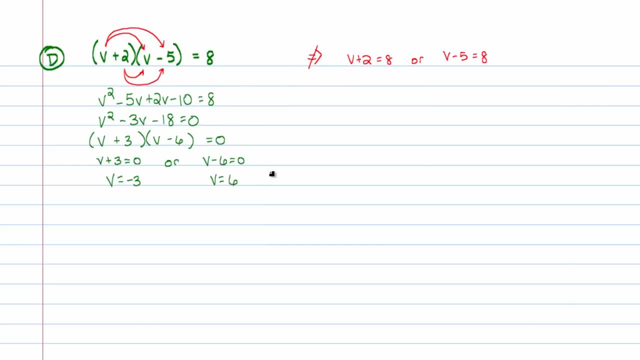 in fact, let me go even back further. Let's see, This is from a previous lecture, but this is good enough. Notice that when you solve a quadratic equation, you start with a quadratic equation. Let's just focus in on this part, right here. 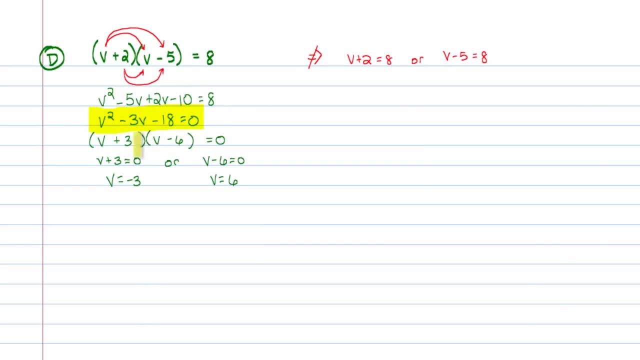 And then you try to factor it and you get down to this beautiful factorization, And then you say: well, either the first object is zero or the second object is zero, which means that v is equal to negative three, or v is equal to six. 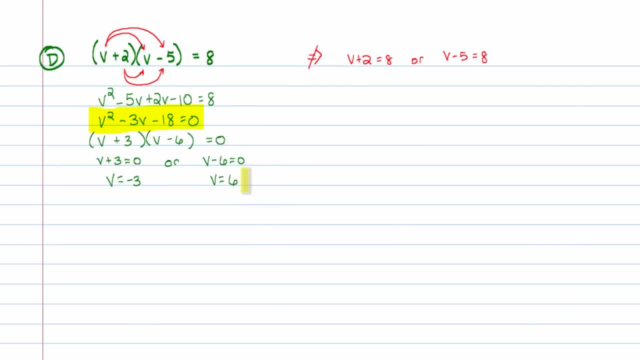 What we did in our last example that we just did here is that we started with this bottom sentence: X is equal to, or, in other words, v is equal to negative three or v is equal to six. Move everything to one side. 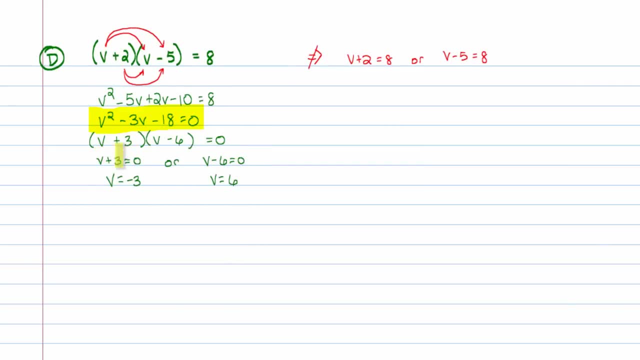 so v minus six is equal to zero, or v plus three is equal to zero. Well, if one of these two has to be zero, then their product must be zero, And if you multiply these things together, you get the original quadratic equation. 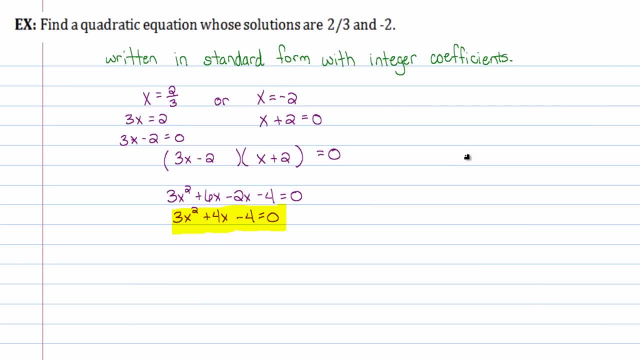 So I want to point out one thing here: That in this process there was a step in here that I kind of did a little bit of hand waving here At this step right here, where I said: oh, x is equal to two thirds. 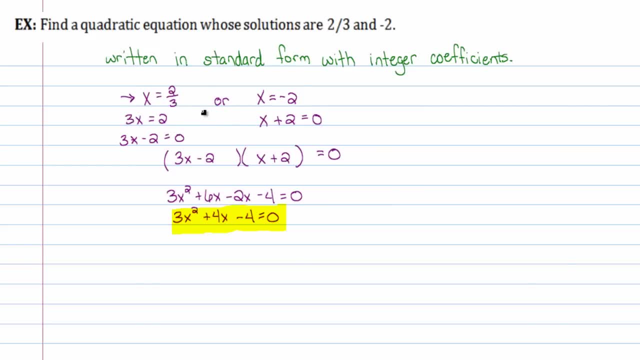 because they told me that's the solution. where x is equal to negative two, I said: multiply both sides by three to get rid of the fraction. If you didn't, you would get this: X minus two thirds is equal to zero. or x plus two is equal to zero. 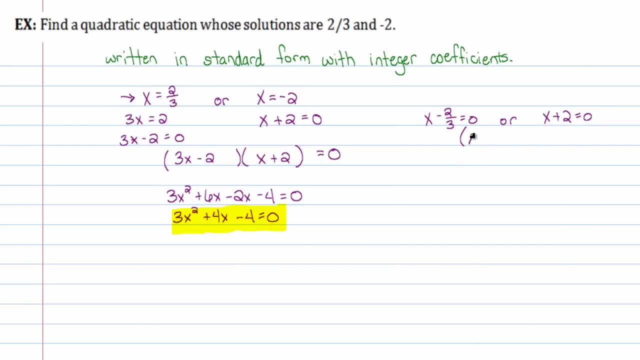 which is fine. If one of these is zero, then x minus two thirds times x plus two would have to be zero. But if you multiply this out, you're not going to get integer coefficients. You're actually going to get rational coefficients.